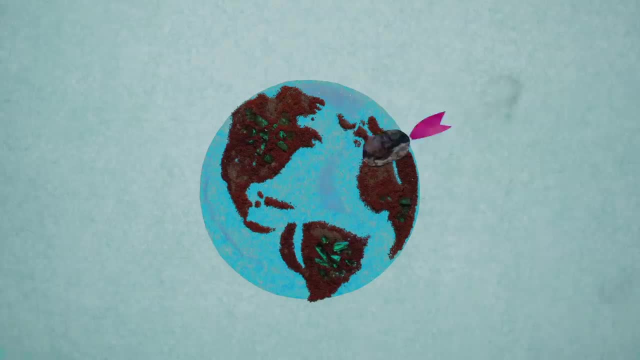 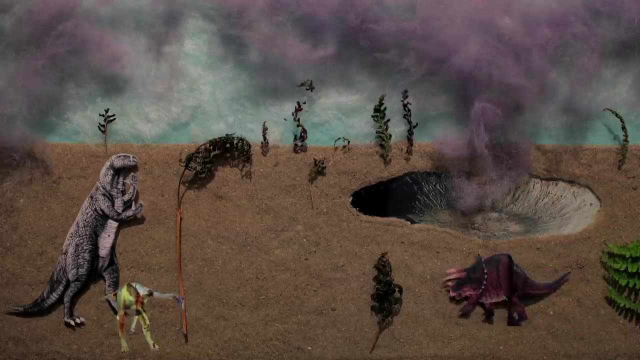 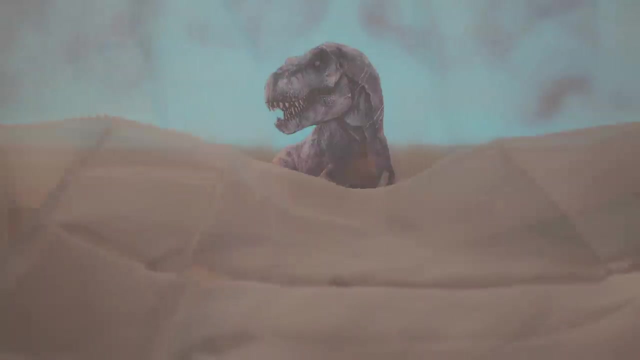 and an asteroid roughly the size of Manhattan struck the Earth. The dust from the impact reduced or stopped photosynthesis for many plants, the starving herbivores and the carnivores that preyed on them. Within a short time span, three-quarters of the world's species disappeared forever. 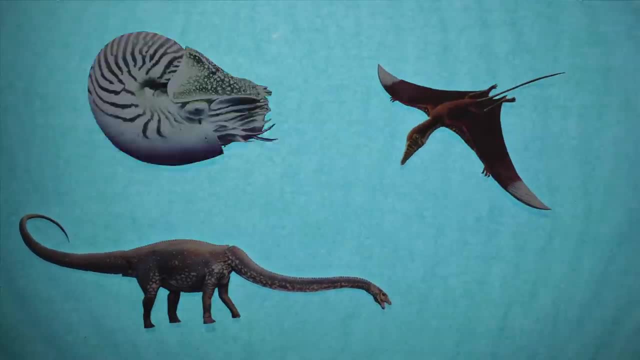 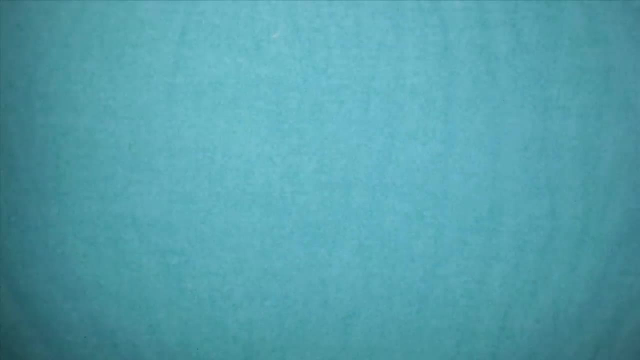 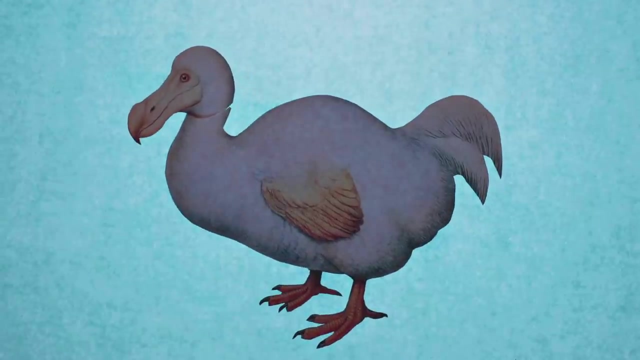 and the giant dinosaurs, flying pterosaurs, shelled squids and marine reptiles that had flourished for ages faded into prehistory. It may seem like the dinosaurs were especially unlucky, but extinctions of various severities have occurred throughout the Earth's history. 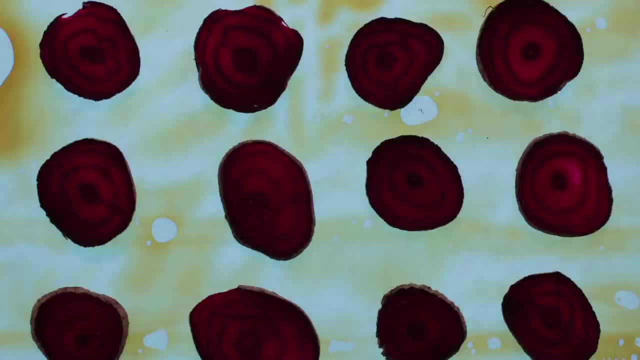 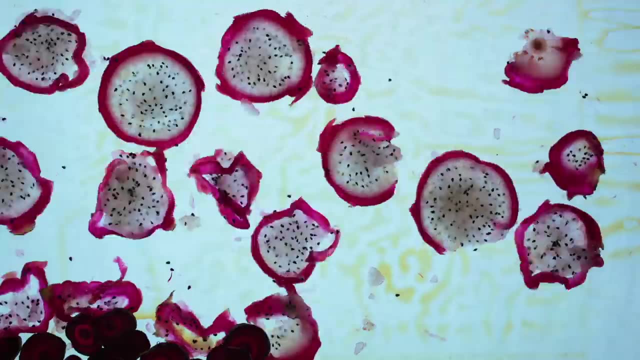 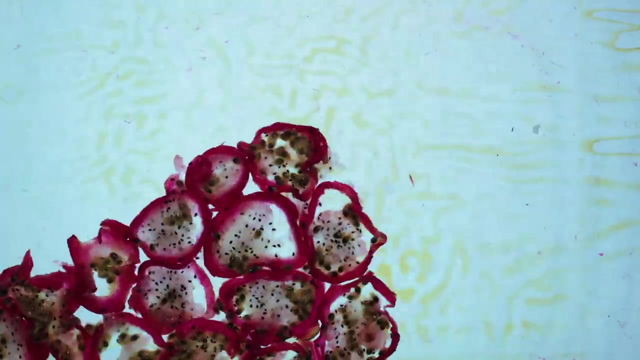 and are still happening all around us today. Environments change, pushing some species out of their comfort zones while creating new opportunities for others. Invasive species arrive in new habitats, out-competing the natives, And in some cases, entire species are wiped out. 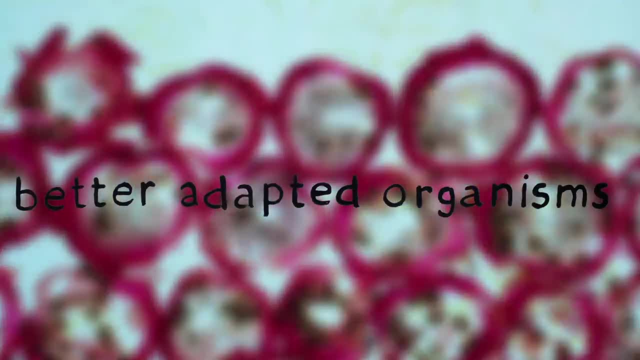 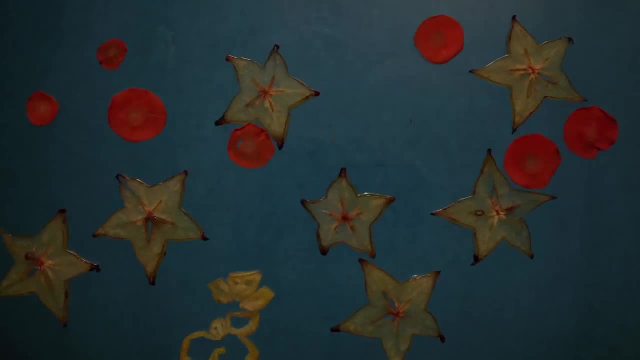 as a result of activity by better adapted organisms. Sometimes, however, massive changes in the environment occur too quickly for most living creatures to adapt, causing thousands of species to die off in a geological instant. We call this a mass extinction event, And although such events may be rare, 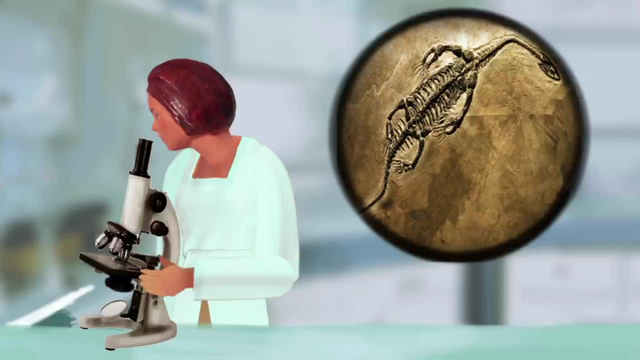 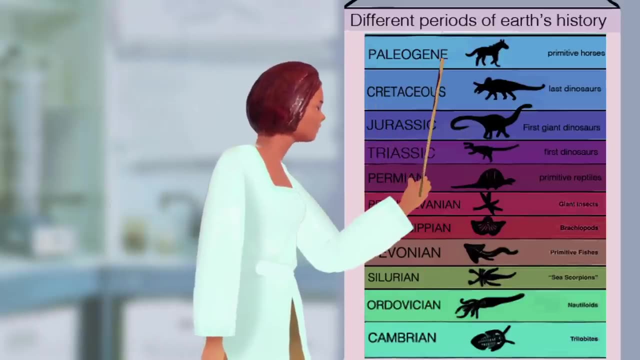 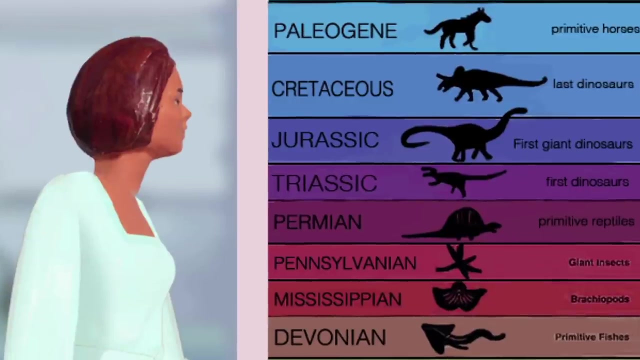 paleontologists have been able to identify several of them through dramatic changes in the fossil record, where lineages that persisted through several geological layers suddenly disappear. In fact, these mass extinctions are used to divide the Earth's history into distinct periods, Although the disappearance of the dinosaurs is the best-known. 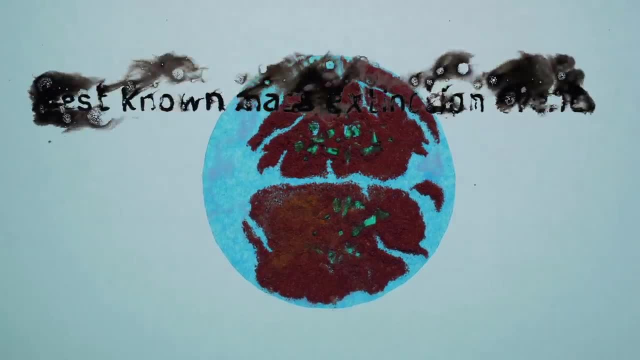 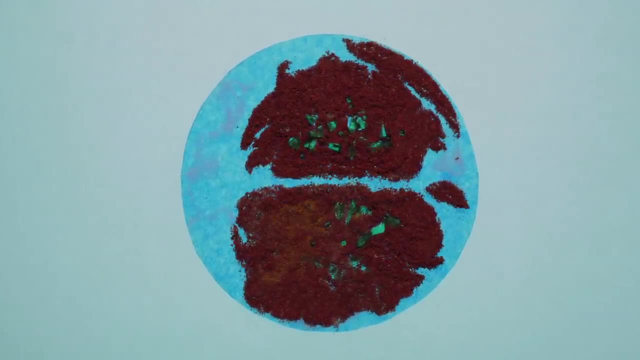 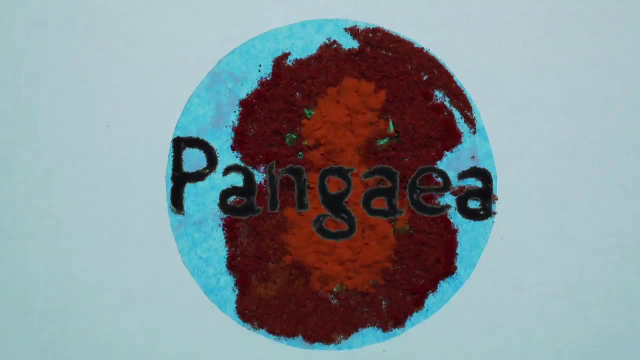 mass extinction event, the largest occurred long before dinosaurs ever existed. 252 million years ago, between the Permian and Triassic periods, the Earth's landmasses gathered together into the single supercontinent Pangea. As it coalesced, its interior was filled with deserts. 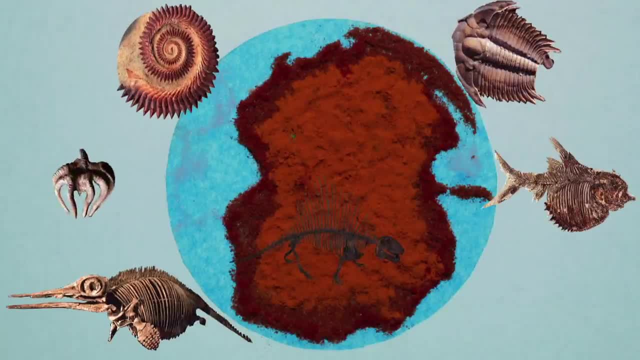 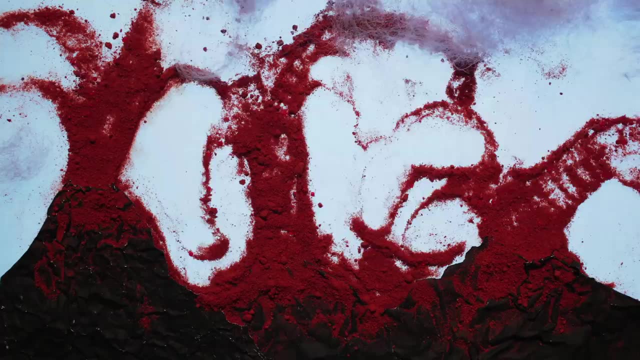 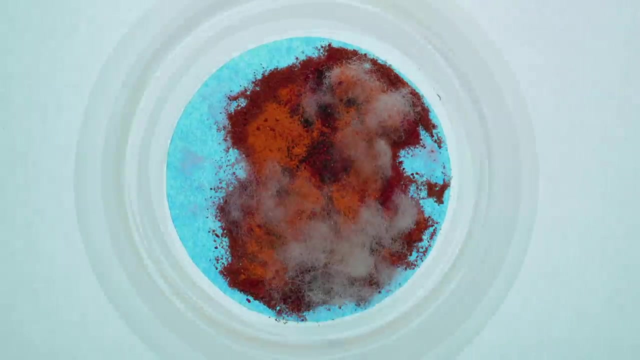 while the single coastline eliminated many of the shallow tropical seas where biodiversity thrived. Huge volcanic eruptions occurred across Siberia, coinciding with very high temperatures, suggesting a massive greenhouse effect. These catastrophes contributed to the extinction of 95% of species in the ocean. 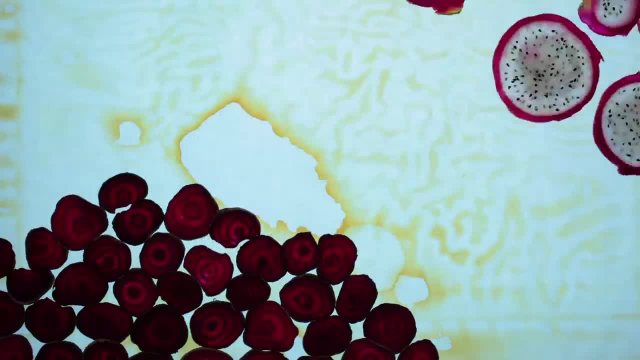 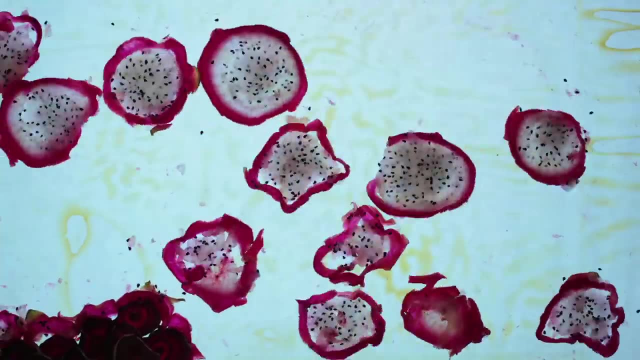 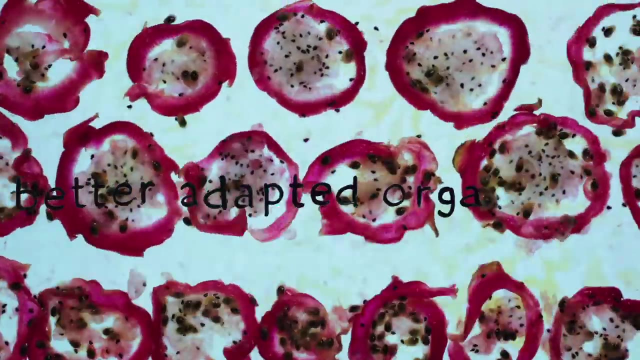 Environments change, pushing some species out of their comfort zones while creating new opportunities for others. Invasive species arrive in new habitats, out-competing the natives, And in some cases, entire species are wiped out as a result of activity by better adapted organisms. 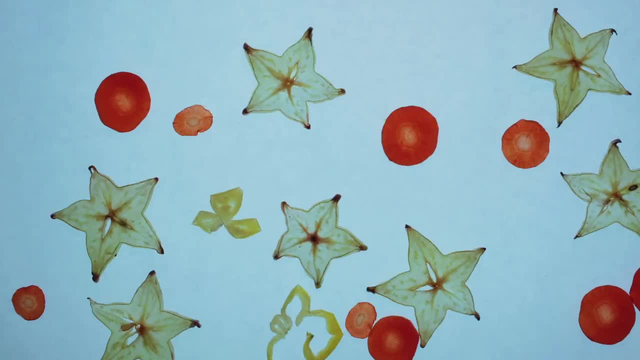 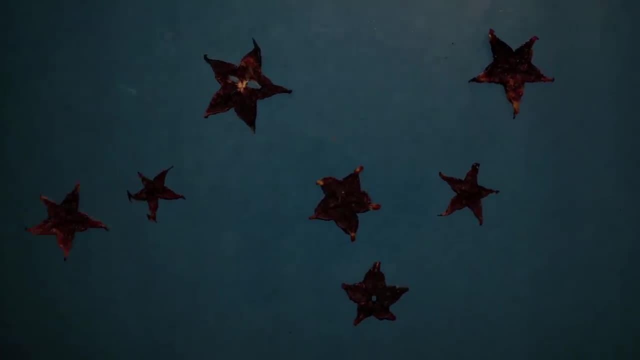 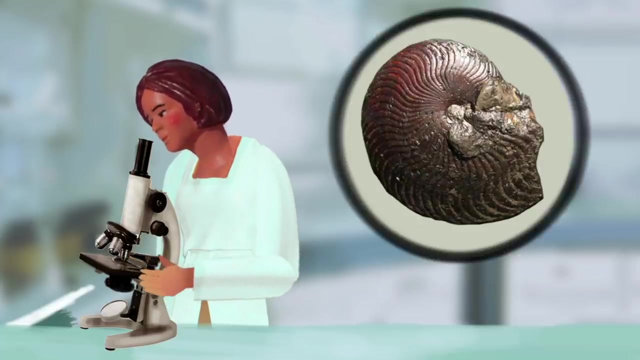 Sometimes, however, massive changes in the environment occur too quickly for most living creatures to adapt, causing thousands of species to die off in a geological instant. We call this a mass extinction event, And although such events may be rare, paleontologists have been able to identify several of them. 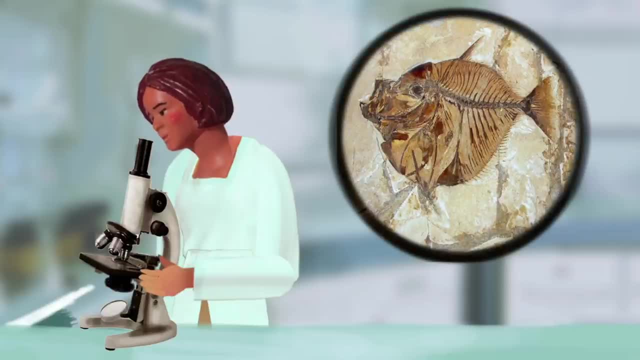 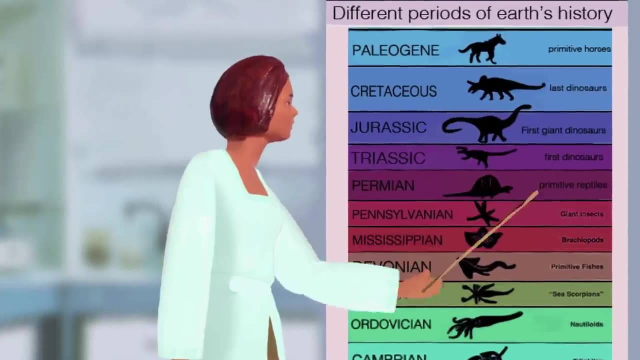 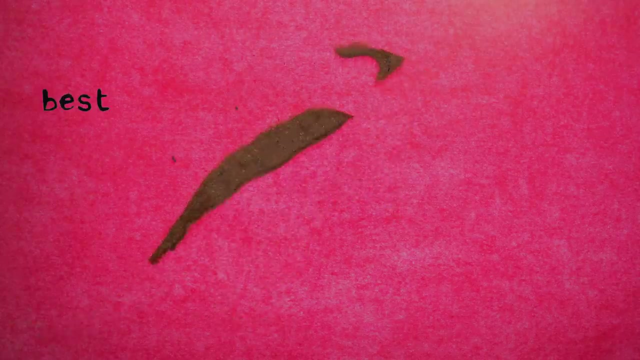 through dramatic changes in the fossil record, where lineages that persisted through several geological layers suddenly disappear. In fact, these mass extinctions are used to divide the Earth's history into distinct periods, Although the disappearance of the dinosaurs is the best-known mass extinction event. the largest occurred long before dinosaurs ever existed. 252 million years ago, between the Permian and Triassic periods, the Earth's landmasses gathered together into the single supercontinent Pangea. As it coalesced, its interior was filled with deserts. while the single coastline eliminated many of the shallow tropical seas where biodiversity thrived. Huge volcanic eruptions occurred across Siberia, coinciding with very high temperatures, suggesting a massive greenhouse effect. These catastrophes contributed to the extinction of 95% of species in the ocean. 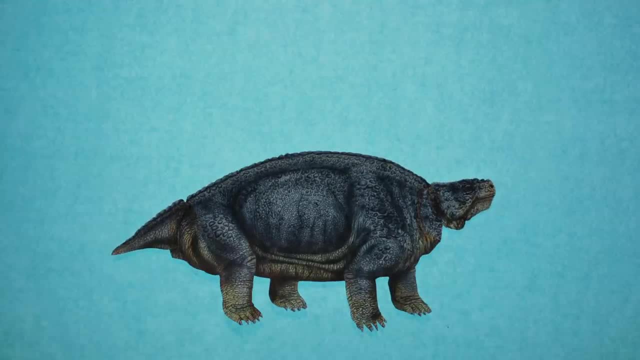 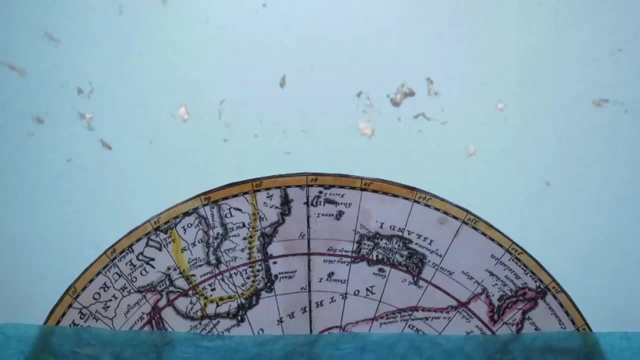 and on land, the strange reptiles of the Permian gave way to the ancestors of the far more familiar dinosaurs we know today. But mass extinctions are not just a thing of the distant past. But mass extinctions are not just a thing of the distant past. 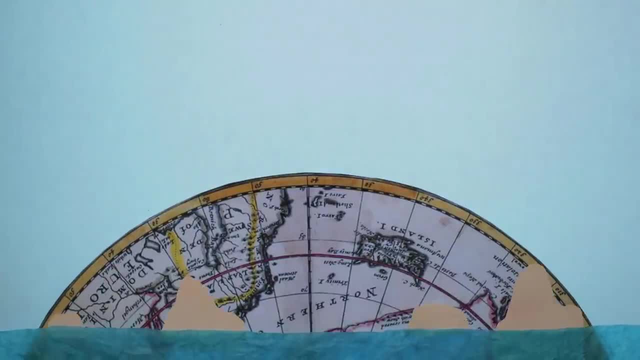 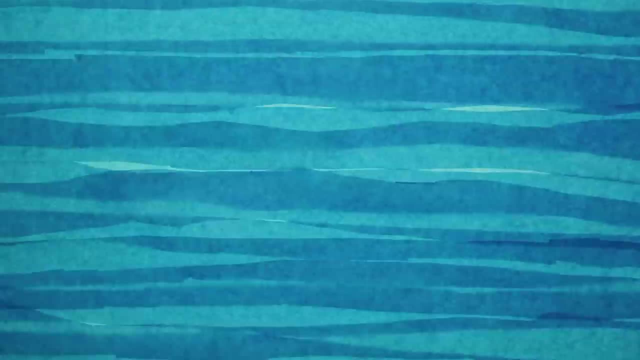 But mass extinctions are not just a thing of the distant past. Over the last few million years, the fluctuation of massive ice sheets at our planet's poles has caused sea levels to rise and fall, changing weather patterns and ocean currents along the way. 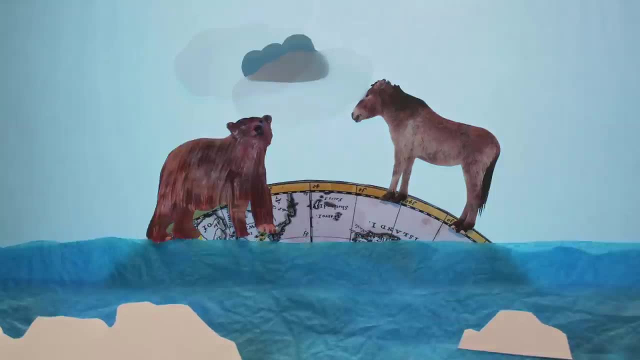 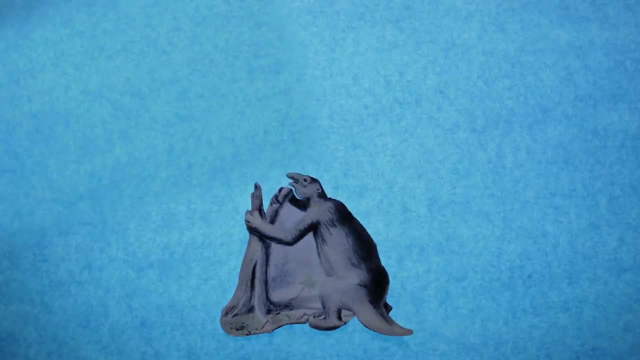 As the ice sheets spread, retreated and returned. some animals were either able to adapt to the changes or migrate to a more suitable environment. Others, however, such as giant ground sloths, giant hyenas and mammoths, went extinct. 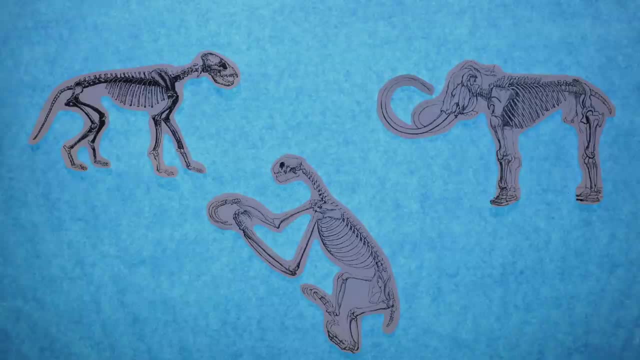 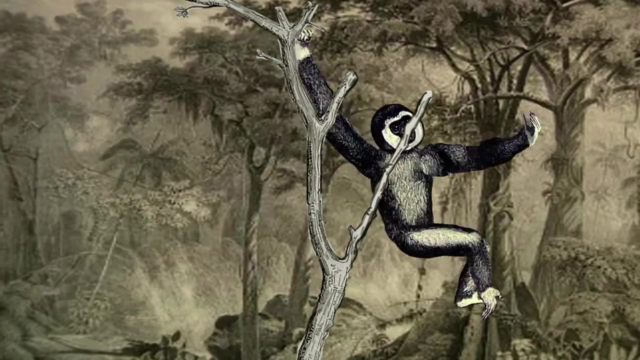 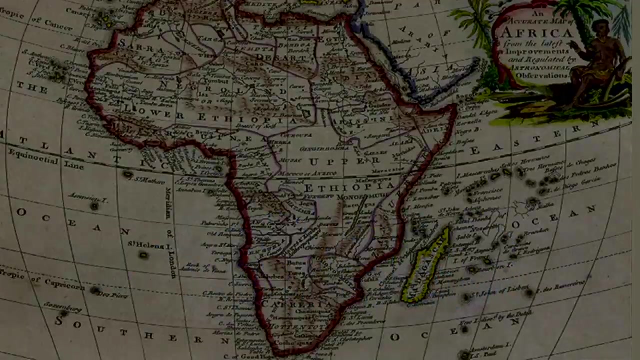 The extinction of these large mammals coincides with changes in the climate and ecosystem due to the melting ice caps, But there is also an uncomfortable overlap with the rise of a certain hominin species originating in Africa 150,000 years ago, In the course of their adaptation to the new environment. 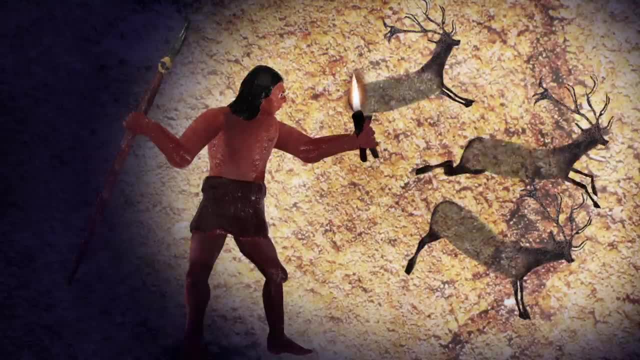 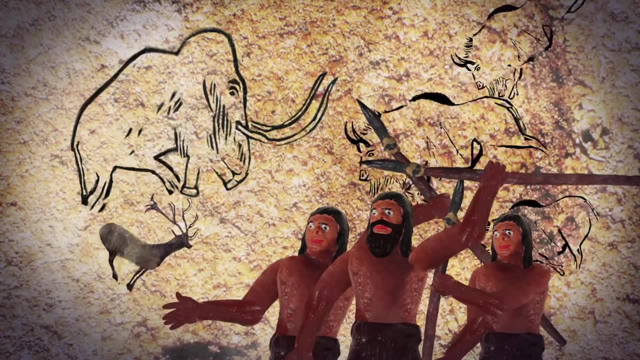 creating new tools and methods for gathering food and hunting prey. humans may not have single-handedly caused the extinction of these large animals. humans may not have single-handedly caused the extinction of these large animals, and some were able to coexist with us for thousands of years. 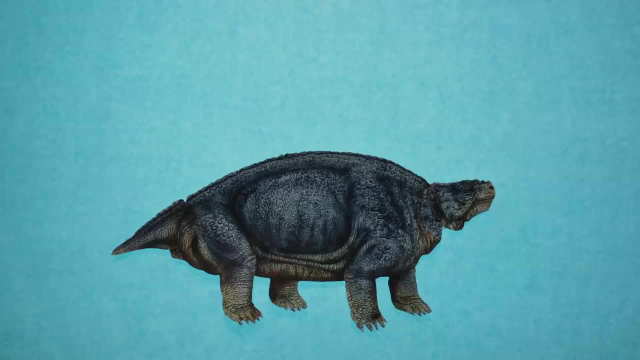 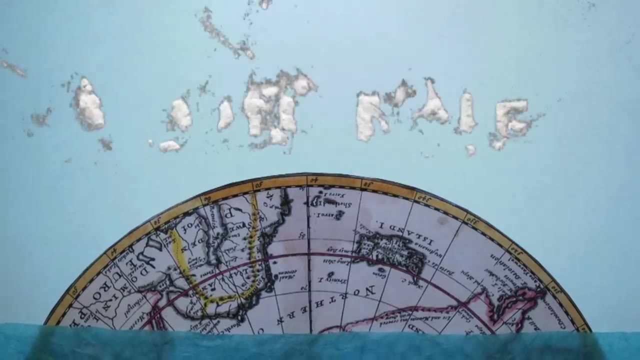 And on land, the strange reptiles of the Permian gave way to the ancestors of the far more familiar dinosaurs we know today. But mass extinctions are not just a thing of the distant past. Over the last few million years, the fluctuation of massive ice sheets 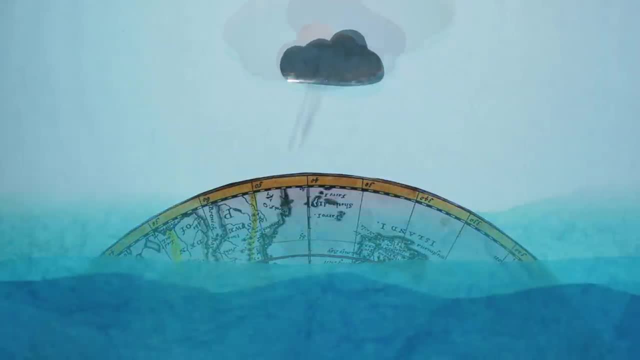 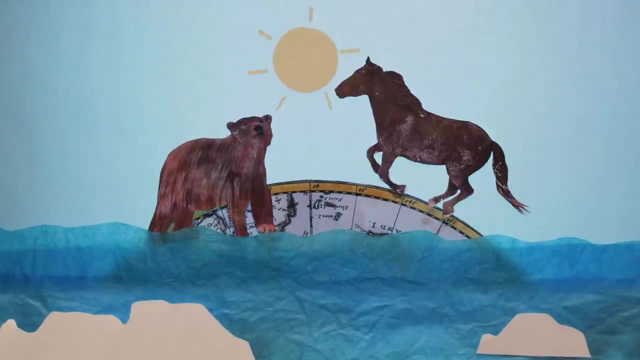 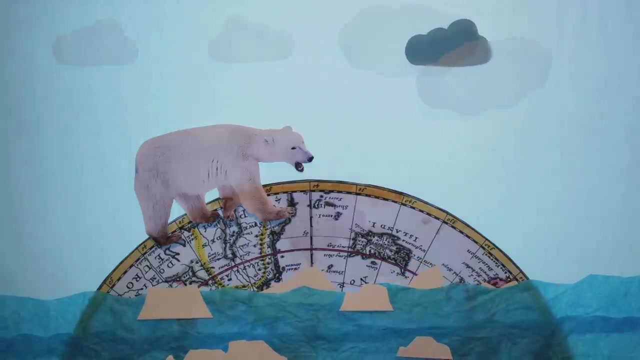 at our planet's poles has caused sea levels to rise and fall, changing weather patterns and ocean currents along the way. As the ice sheets spread, retreated and returned, some animals were either able to adapt to the changes or migrate to a more suitable environment. 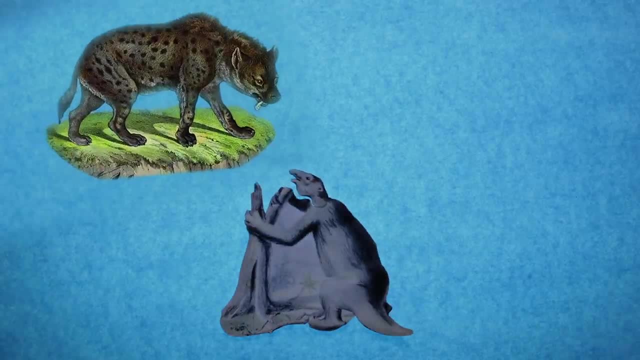 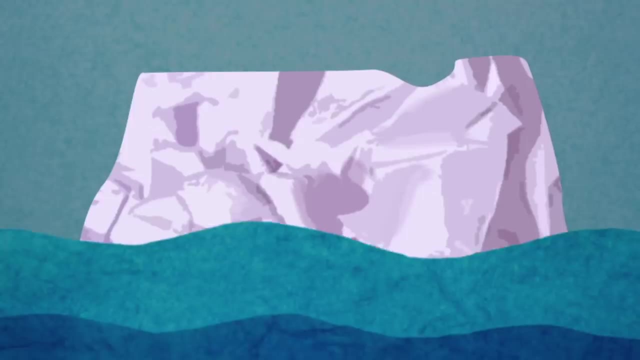 Others, however, such as giant ground sloths, giant hyenas and mammoths, went extinct. The extinction of these large mammals coincides with changes in the climate and ecosystem due to the melting ice caps, But there is also an uncomfortable overlap. 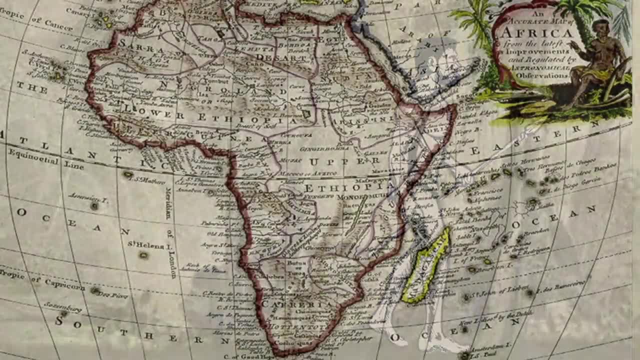 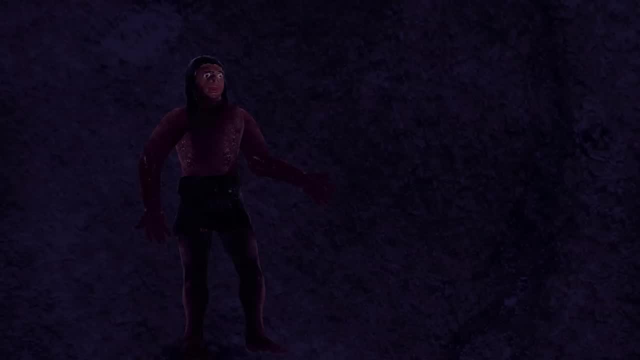 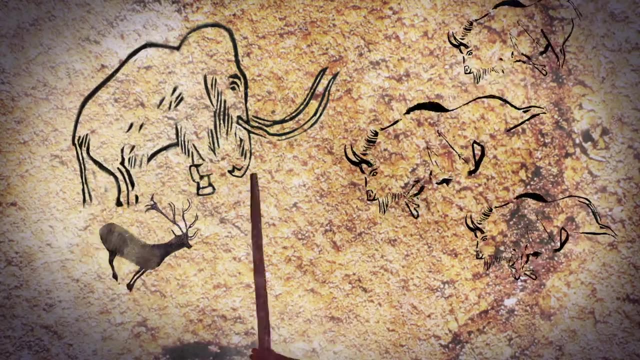 with the rise of a certain hominin species originating in Africa 150,000 years ago, In the course of their adaptation to the new environment, creating new tools and methods for gathering food and hunting prey. humans may not have single-handedly caused the extinction of these large animals. 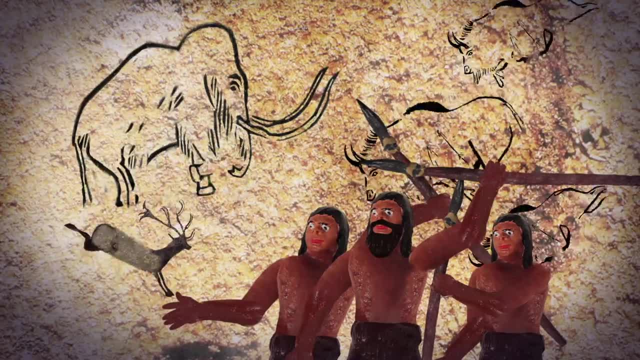 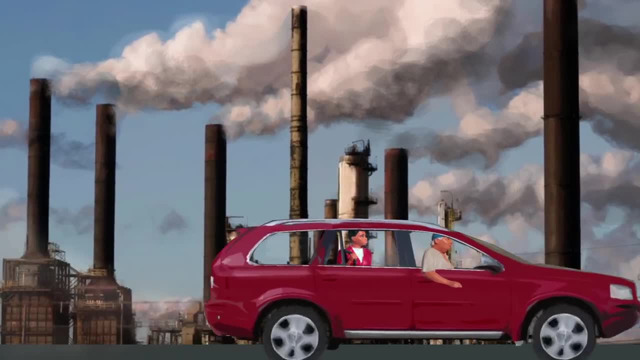 as some were able to coexist with us for thousands of years. But it's clear that today our tools and methods have become so effective that humans are no longer reacting to the environment, but are actively changing it. The extinction of species is a normal occurrence. 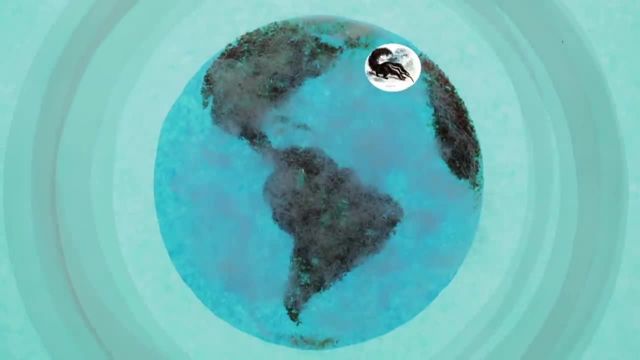 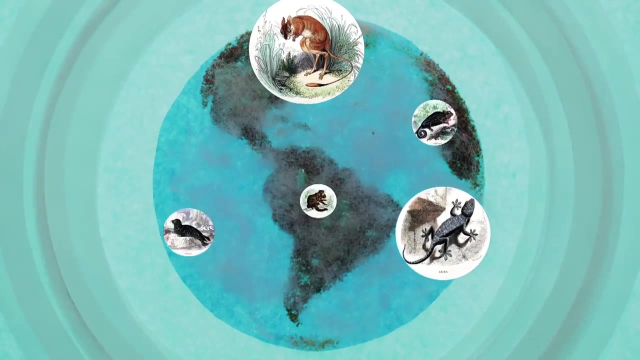 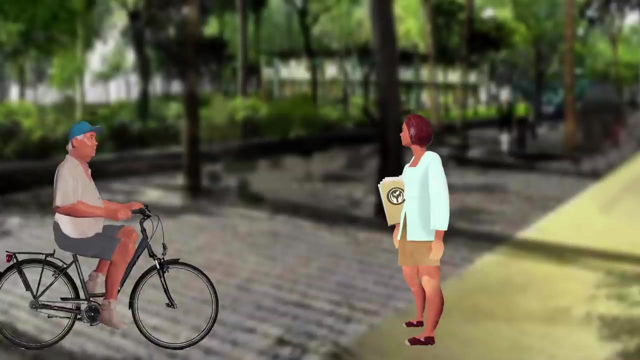 in the background of ecosystems, But studies suggest that rates of extinction today for many organisms are hundreds to thousands of times higher than the normal background. But the same unique ability that makes humans capable of driving mass extinctions can also enable us to prevent them. 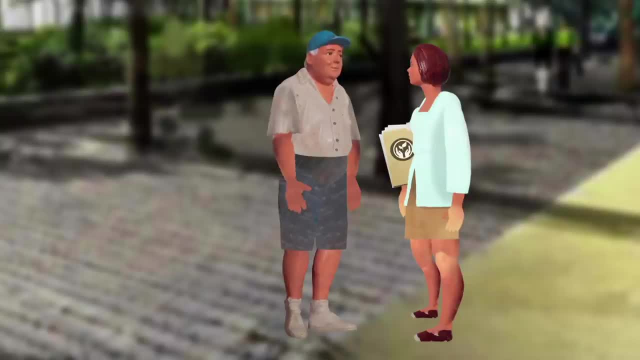 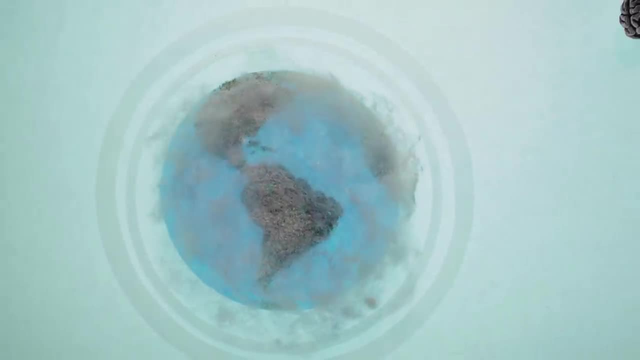 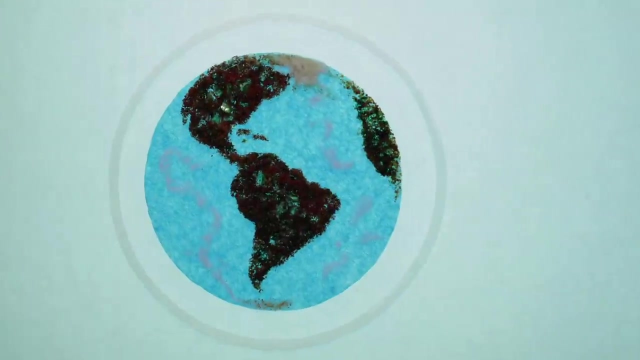 By learning about past extinction events, recognizing what is happening today as environments change, and using this knowledge to lessen our effect on other species, we can transform humanity's impact on the world from something as destructive as a massive asteroid into a collaborative part of a biologically diverse future. Transcription by ESO. Translation by —. 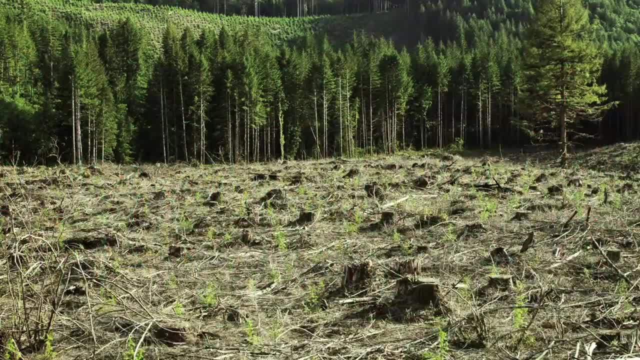 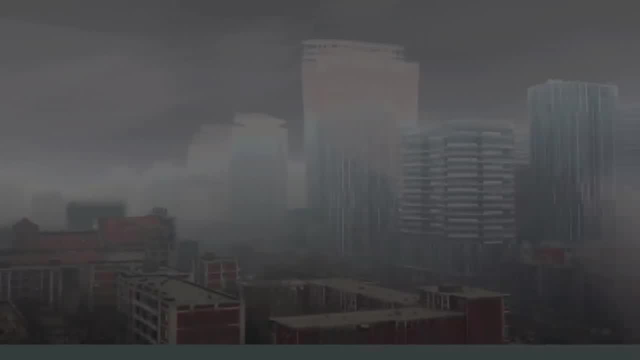 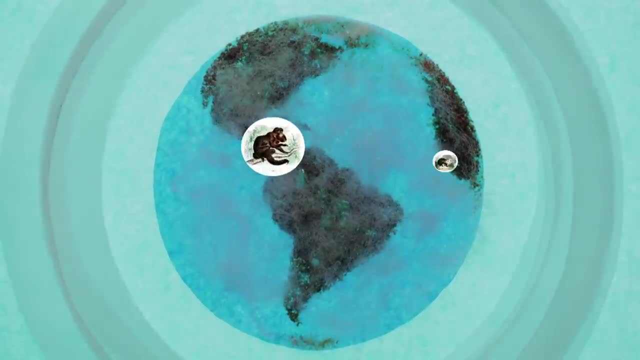 But it's clear that today our tools and methods have become so effective that humans are no longer reacting to the environment but are actively changing it. The extinction of species is a normal occurrence in the background of ecosystems, but studies suggest that rates of extinction today for many organisms 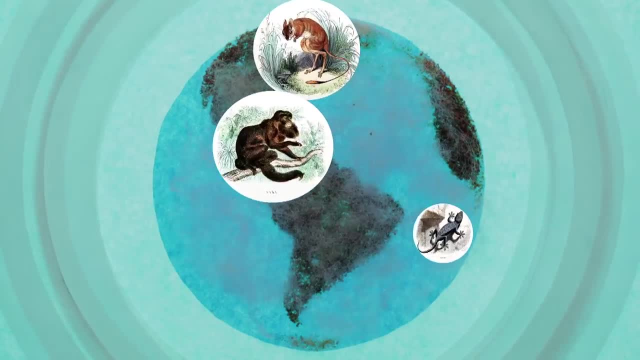 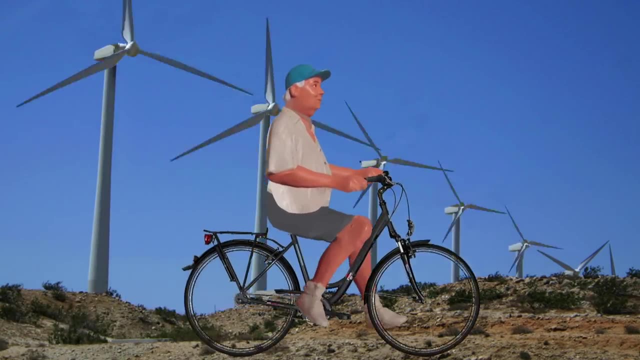 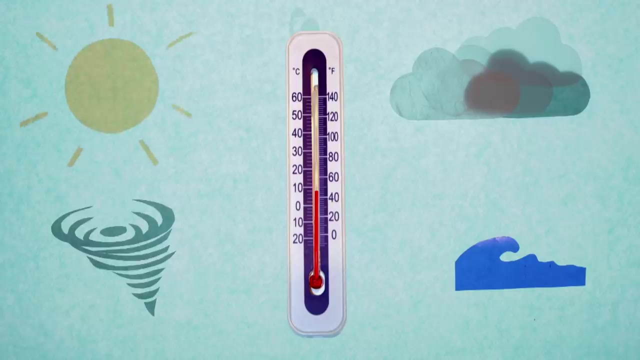 are hundreds to thousands of times higher than the normal background. But the same unique ability that makes humans capable of driving mass extinctions can also enable us to prevent them By learning about past extinction events, recognizing what is happening today as environments change, and using this knowledge to lessen our effect on other species. 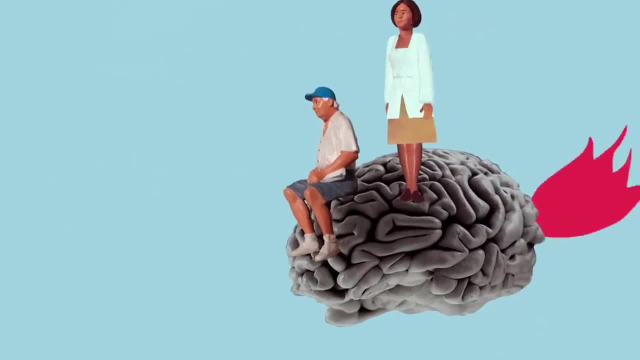 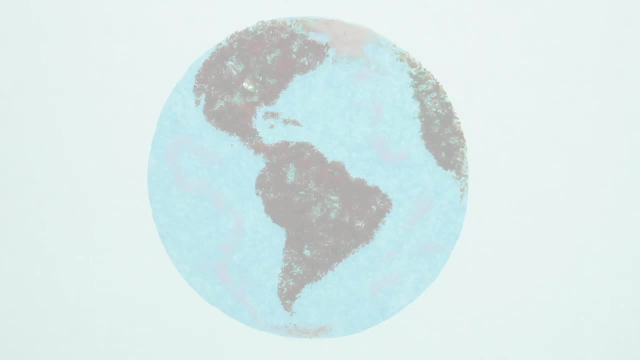 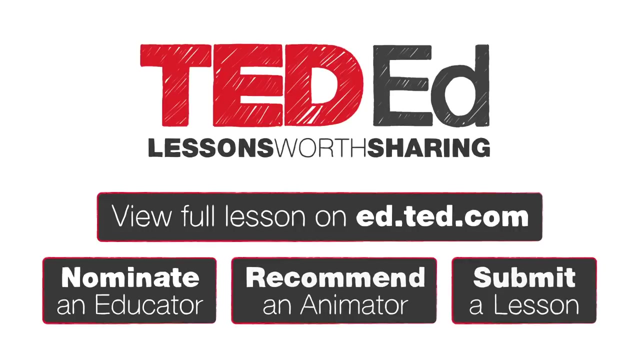 we can transform humanity's impact on the world from something as destructive as a massive asteroid into a collaborative part of a biologically diverse future. Subtitles by the Amaraorg community. 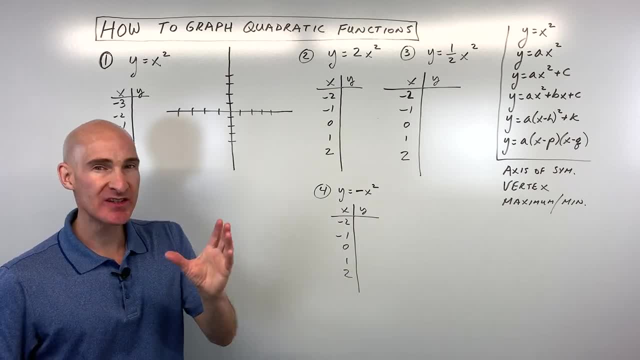 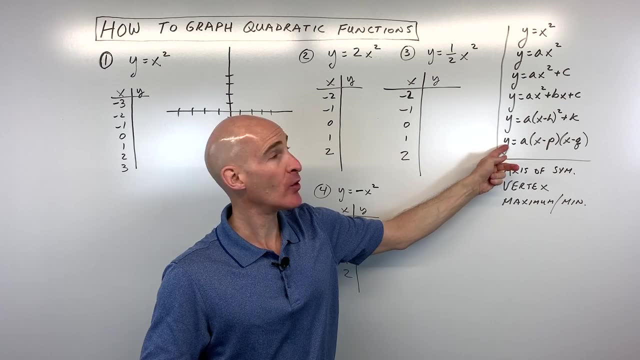 In this lesson you're going to learn how to graph quadratic equations. These are the parabola-shaped graphs, And what we're going to do is we're going to work through all these different forms of the quadratic equation here to graph these parabolas in these different 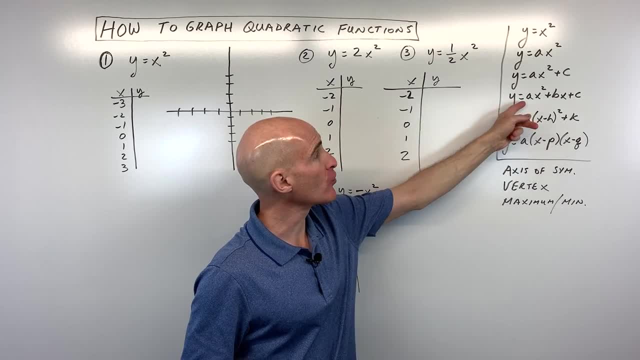 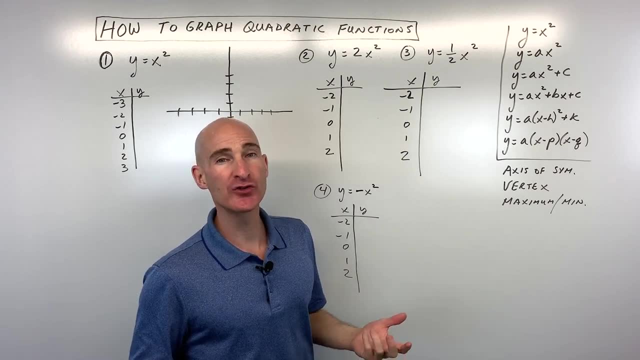 forms. So we've got the vertex form, the intercept form, the standard form and then some of the parent function graphs. We're also going to talk about transformations and we're going to talk about how to approach these graphs so you can easily get a good graph. So let's. 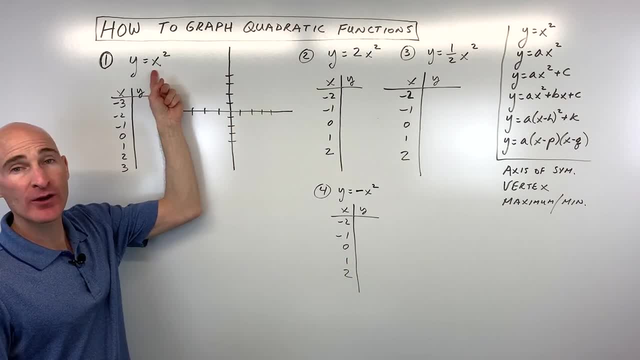 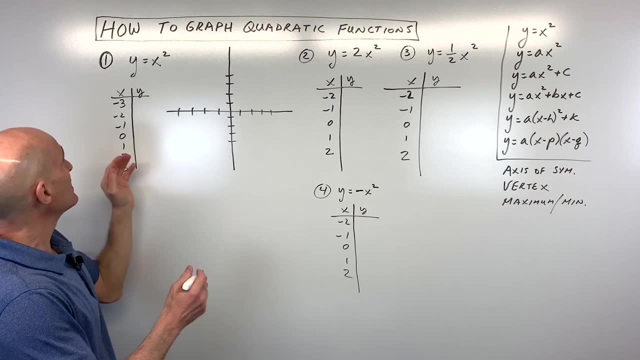 dive in. The first problem is just to basically look at the y equals x squared form of the equation, And this is what we call our parent function. What you can do is you can just pick some points. I usually pick a couple negative, zero and a couple positive, And